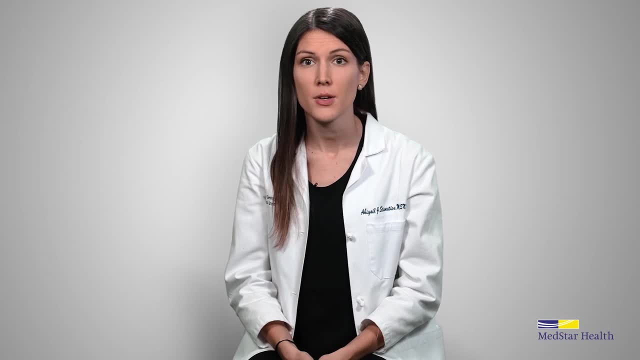 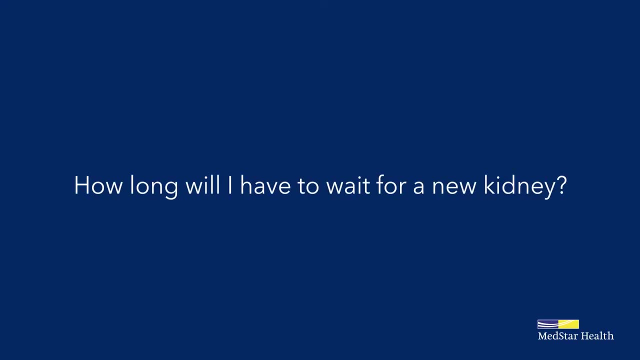 operated by the United Network of Organ Sharing, or UNOS. UNOS is a national organization for organ allocation. Wait time for a donor organ is dependent upon several factors. These include your blood type and tissue matching. Expected patient waiting times vary depending upon your. location within the US, as well as the local organ procurement organization or OPO, For AB blood types. you need to have a donor organ. You need to have a donor organ. You need to have a blood type. the wait time is typically less than two years. Blood type A: about three to five years. 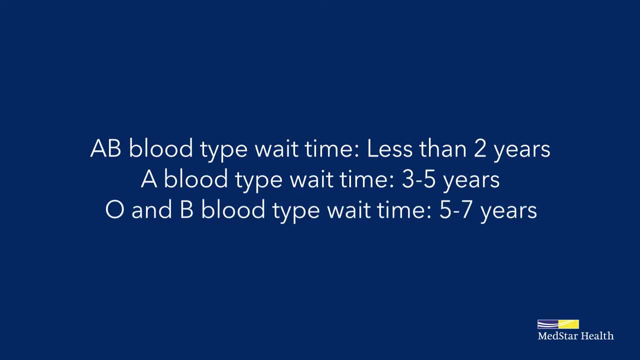 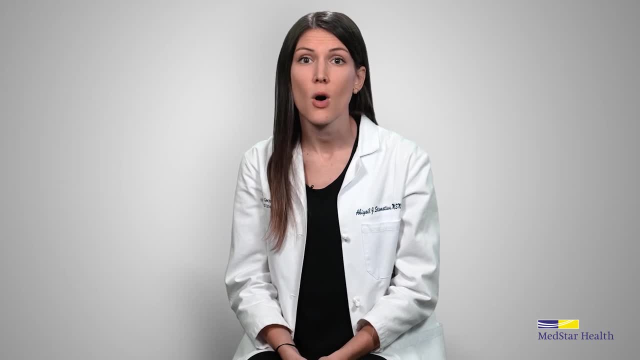 and for other blood types, O and B, typically five to seven years. If you have a living donor that is approved, the transplant can be scheduled within a few months. so we encourage all our patients to look for a living donor to greatly shorten their wait time. Wait time may change. so it's very important to look for a living donor. It is important to know your wait time officially starts the day you started dialysis. So if you've been on dialysis for three years, when you get listed you start with three years of wait time right away. 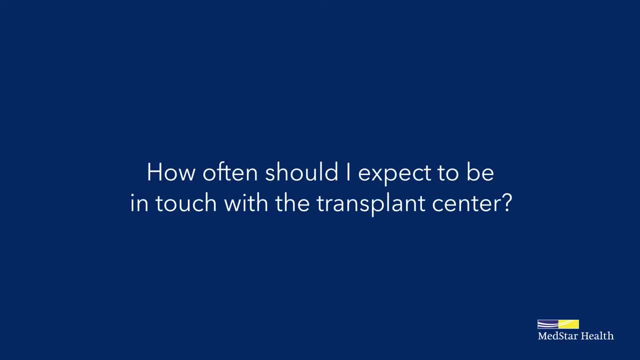 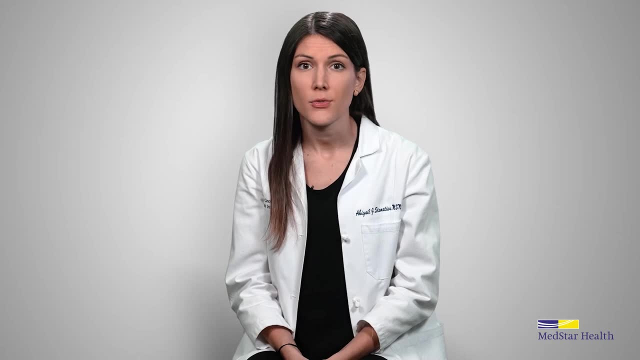 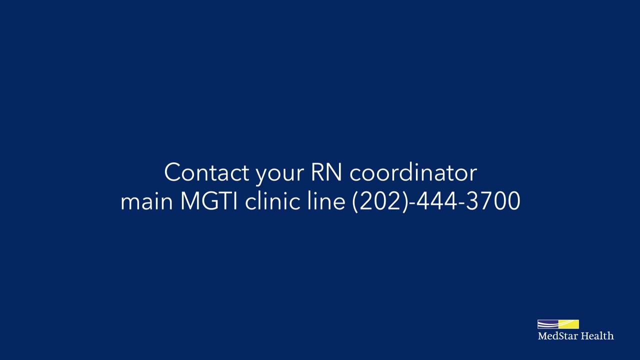 While we may only be in touch with you every six to 12 months, you should always feel free to contact your coordinator while on the waitlist at MGTI at 202-444-3700, and know we will always be in touch with you. We encourage you to save your coordinator's 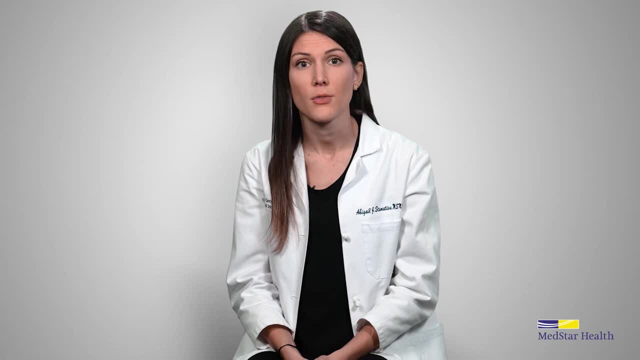 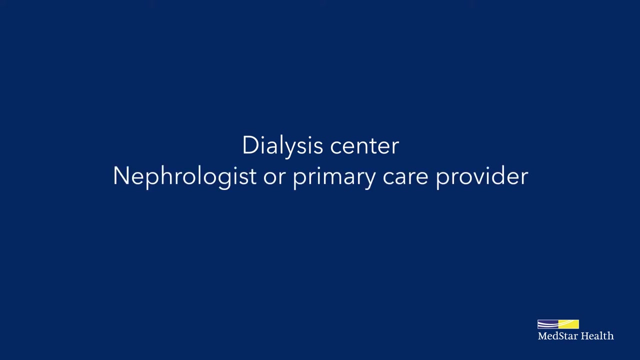 number or the MGTI main clinic number into your cell phone. We need to know about any change in your contact information, including changes to your dialysis center, new nephrologist or primary care provider and any change in insurance information. 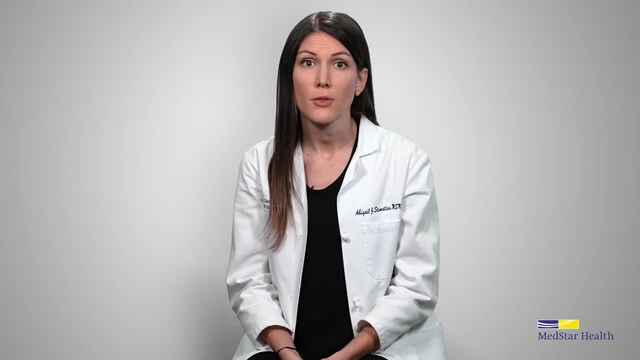 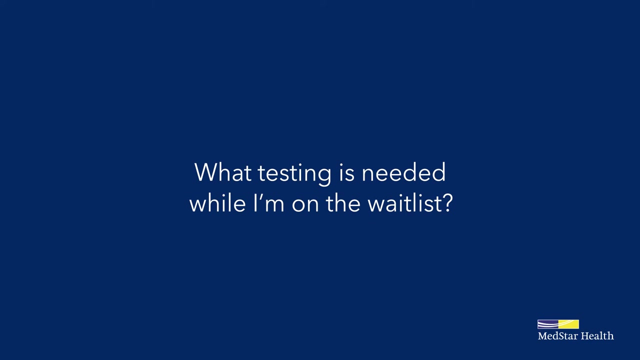 We would like to hear about any and all significant changes to your health condition, including medications and any surgeries. Please do not call or email your coordinator at MGTI Again. the number is 202-444-3700.. The MGTI team will contact your primary nephrologist if there is any change in your health or status. 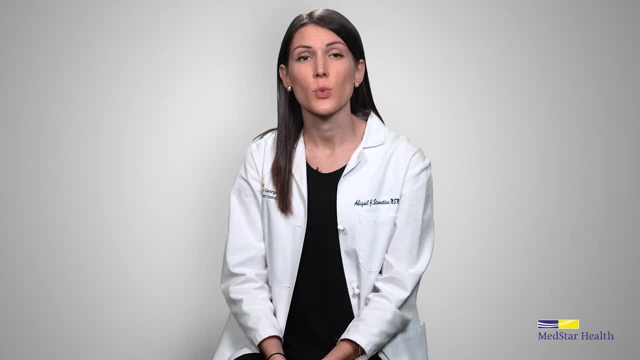 Testing you will need while on the waitlist includes a monthly blood test, which is one red-top tube for PRA testing, which is done to study your immune system. We need a sample of blood sent to our lab every month. you are on the list If we do not have blood. 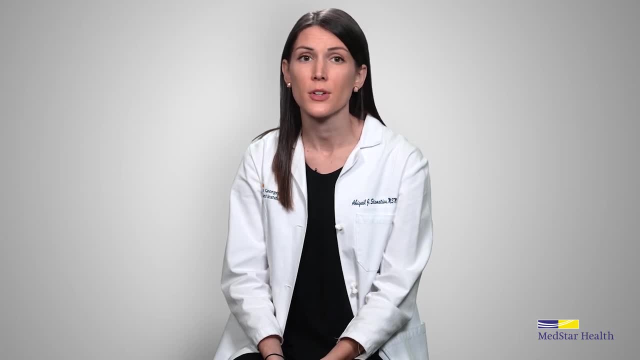 from you, we cannot test the kidneys and you will not be offered a transplant. If you are on dialysis, your monthly PRA kits are done at your dialysis center. Notify your coordinator if your dialysis center changes. Non-dialysis patients can choose to. 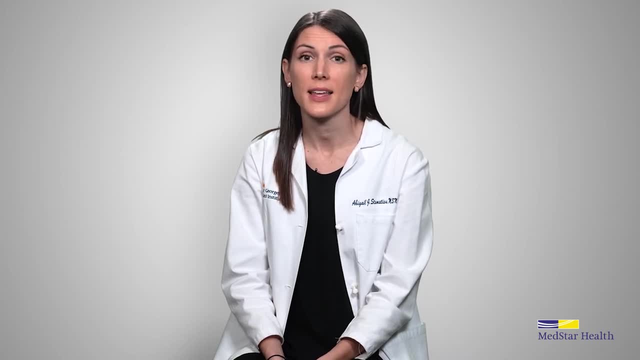 bring their PRA kit to a non-MedStar lab to get this test done. Alternatively, a non-dialysis patient can choose to come to either MedStar, Georgetown University Hospital or Washington Hospital Center to have their monthly PRA lab drawn. They must bring their kit and lab form. 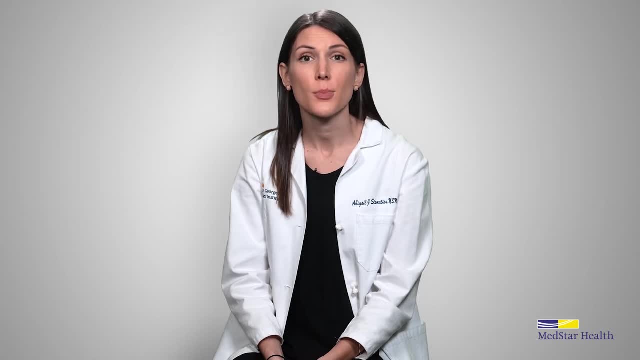 generated by their transplant coordinator. Patients who perform home dialysis can take their kit to the dialysis center when they have their regular in-person visit. This is usually completed monthly. If you have a question about PRA testing, please do not hesitate to ask your. 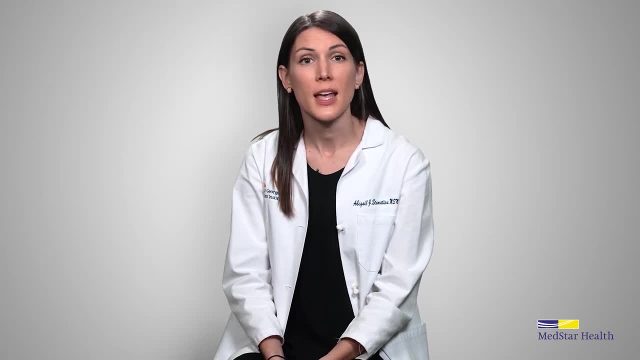 transplant coordinator. Other testing includes annual screening for hepatitis and other viruses. as part of your annual lab work, You also get an annual chest x-ray and EKG, Also repeat heart testing, which includes a stress test and an echocardiogram every one to two years. You also 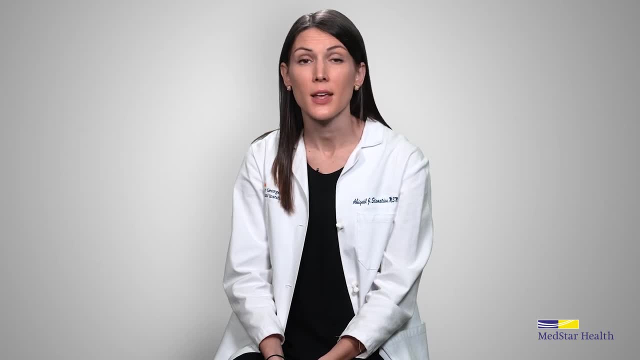 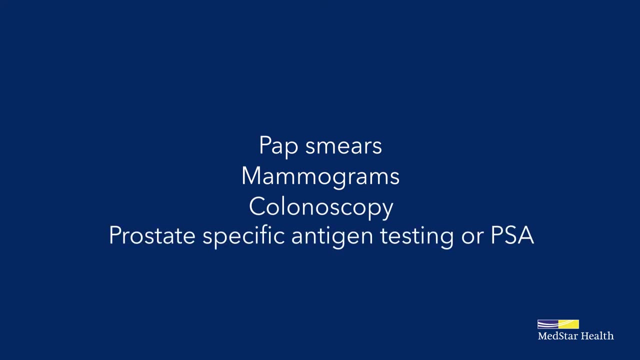 must keep current with standard screening testing including, as appropriate, pap smears, mammograms, colonoscopy and prostate-specific antigen testing, or PSA. This will be explained specifically during your waitlist visit. You should stop using all tobacco products. 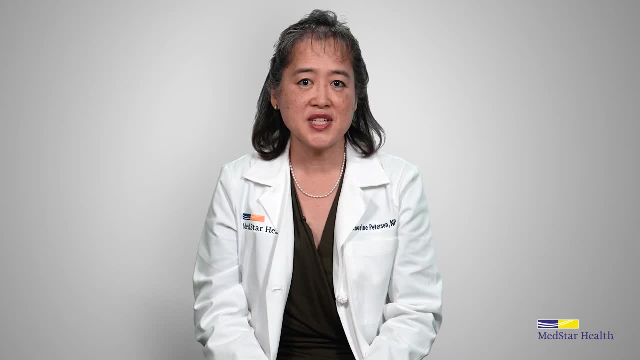 cigarettes, cigars, pipes and dip. Some studies have found that people who smoke are eight times more likely to lose the kidney than people who do not smoke. If you are a diabetic, it's very important to keep your kidneys clean. If you are a diabetic, it's very important to keep your kidneys. 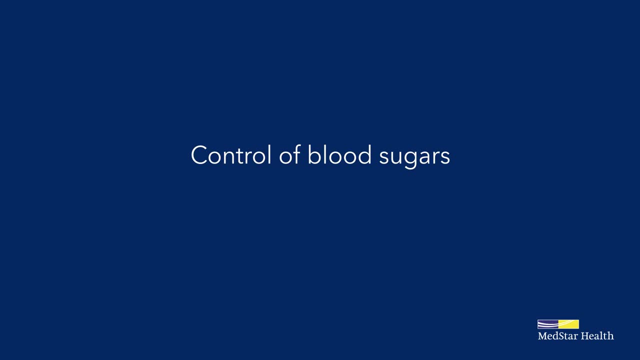 clean. If you are a diabetic, it's very important to have good control of your blood sugars prior to transplant. Keep your weight well controlled, because risks increase for patients who are overweight. It's important to stay active and exercise regularly so you are able to be strong. 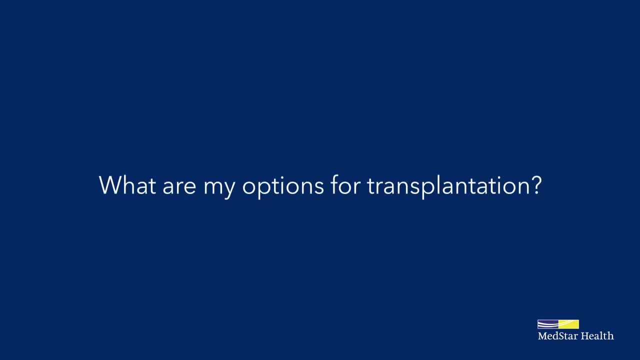 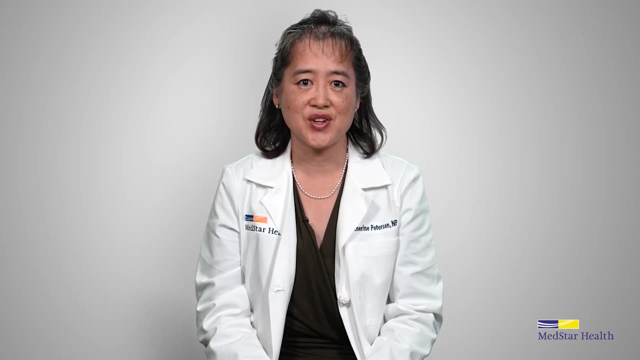 in preparation for your transplant surgery. Patients can receive a kidney either from a living donor or a deceased donor. A living donor is superior to a deceased donor kidney in several ways. Most living donor kidneys function immediately and last an average of 15 to 20 years. 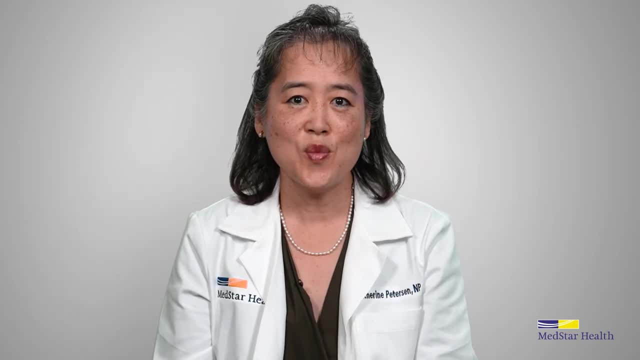 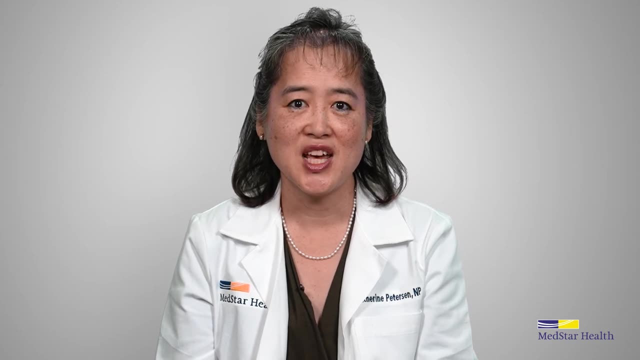 and there is much less wait time for a transplant. We want recipients to always think of any individual that is medically and psychologically able to undergo the donor operation, and the MGTI team will find a kidney for them, either the donor they bring forward or with our expansive and successful PKE program. 70% of deceased donor kidneys function immediately for an average of 10 to 12 years. If you are a diabetic, it's very important to keep your kidneys clean. If you are a diabetic, you'll want more blood sugars but require longer wait times on the list For diabetics. 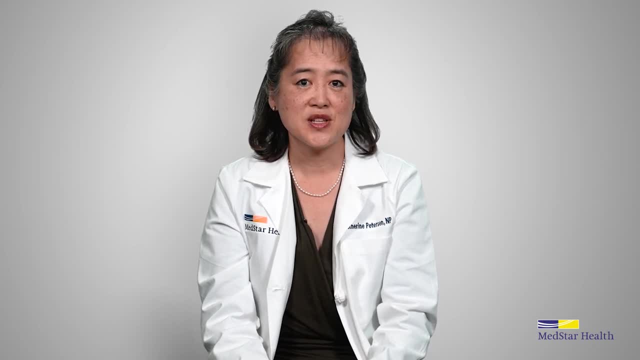 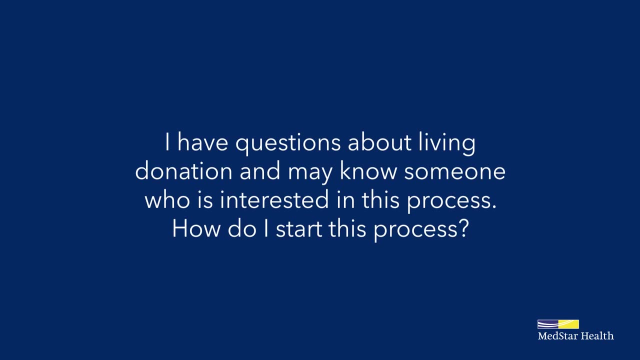 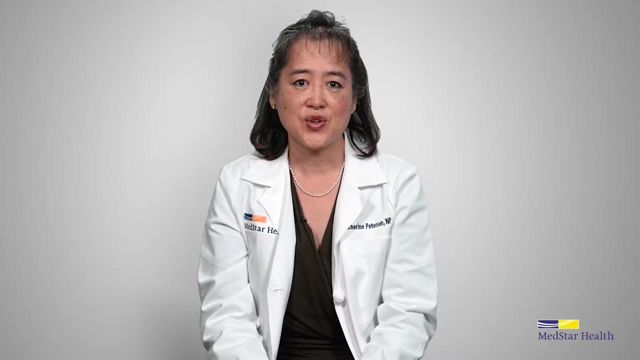 there is an option of pancreas transplant. A few requirements are age, BMI and health status. The first step to being considered as a living donor is for the donor to complete the donor questionnaire at MedStarGeorgetownorg livingkidneydonorcom. After the donor's full medical questionnaire, the donor will be able to have the discarded kidney from the görevolama including their medical information. After receiving a donation, the donor will recall the address and the address of the donor. This will then be referred to as a donor listed. 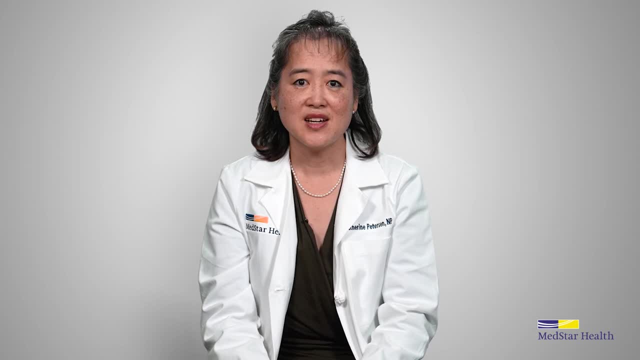 as a living donor. We will give the donor's full name, name and address at medstargeorgetownorg. MedStarGeorgetownorg is also an important place to find those working with kidney and kidney kidney blind. After registration or the questionnaire is completed, someone from MGTI will contact the donor directly. 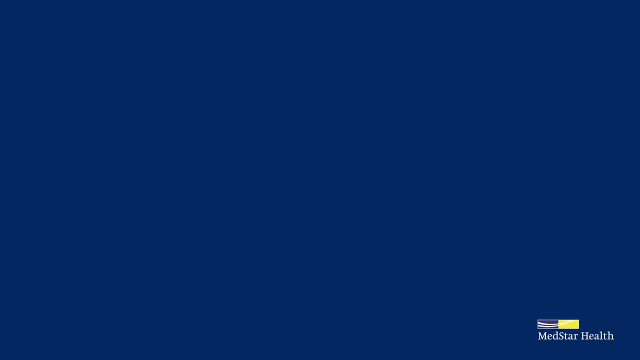 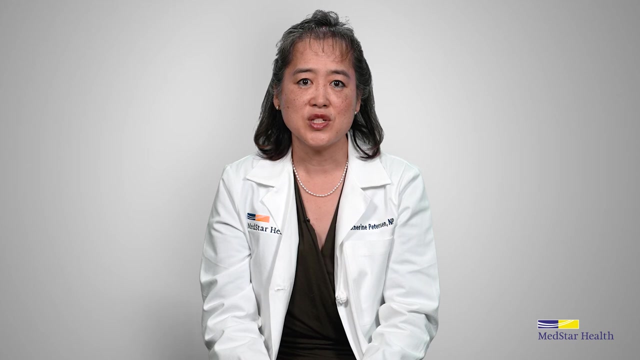 During your waitlist update visit, you'll meet the team, which includes your RN coordinator, financial coordinator, social worker, provider and dietitian. Number one is testing. Let your coordinator know once you've booked your tests and send them results. 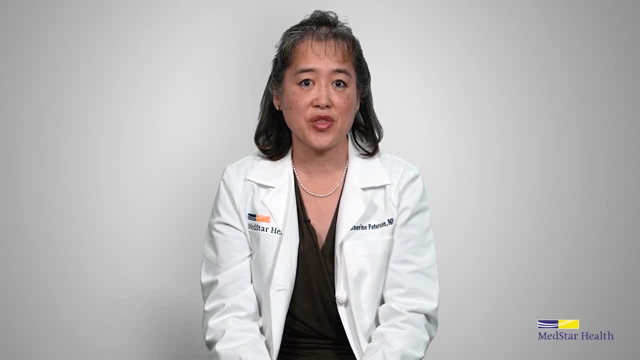 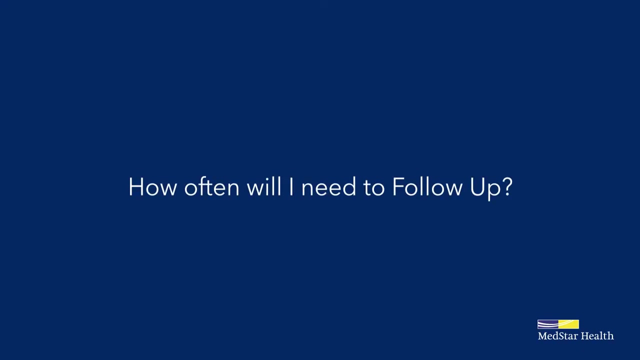 The goal is to have the ordered testing completed within three months of your waitlist visit. You are your best advocate and the work you put into maintaining up-to-date testing helps you to stay active and cleared on the list. You can expect to be seen every year, or twice a year if you're older than 70.. 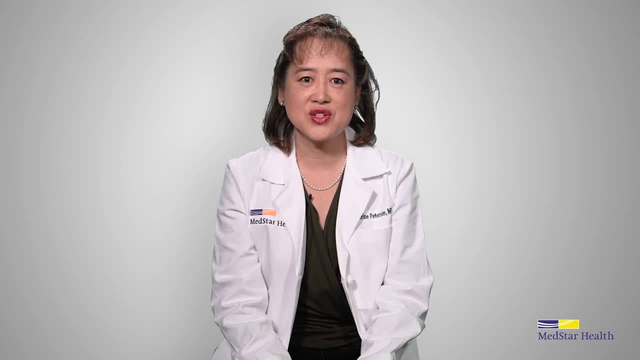 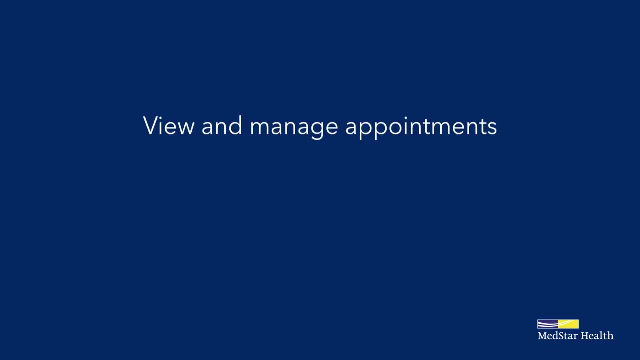 We encourage all patients to enroll in the MUNCH program. This is a free, secure and convenient patient portal where you can keep track of all of your health information 24-7.. With My MedStar, you can view and manage appointments, see test results, renew prescriptions, access your health records and, most importantly, communicate with your provider. It's easy to enroll. You can go directly to mymedstarorg slash enroll. You only need your name, date of birth and your MedStar Health patient ID. Your unique patient ID can be found on the first page of your visit or discharge summary. 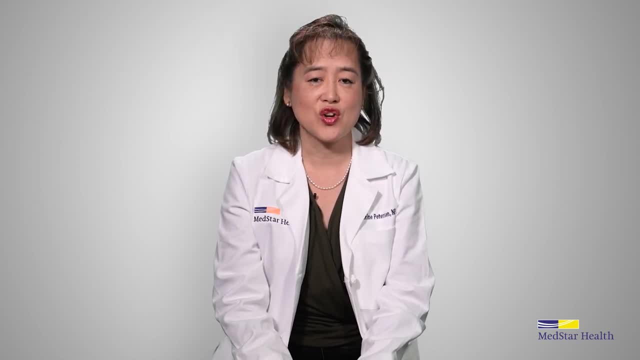 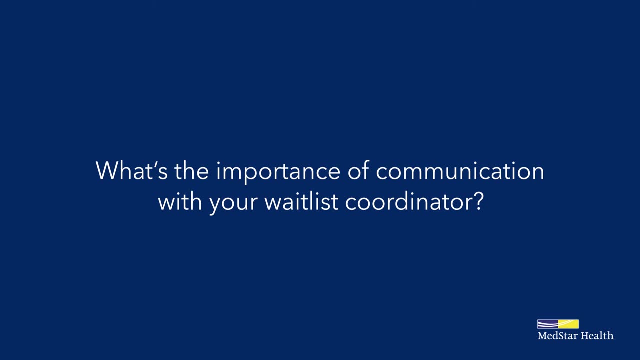 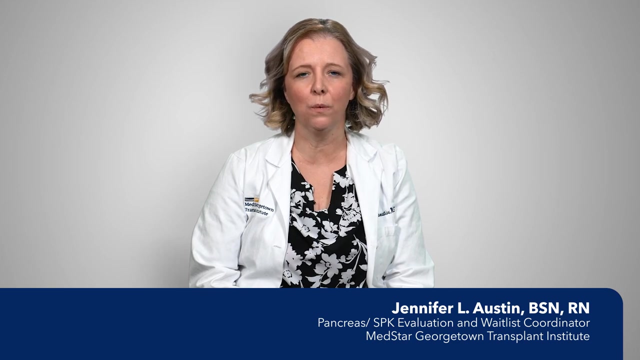 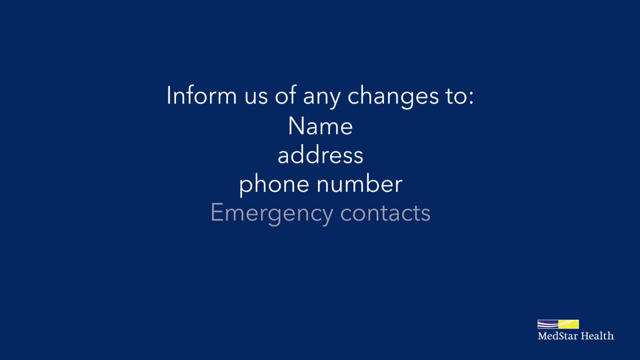 If you don't have your patient ID, ask a MedStar Health associate or complete the secure request form at mymedstarorg slash enroll. Due to the possibly extended wait time for an organ, it is important that you keep in touch with your coordinator and keep them informed of any changes in your name, address, phone number, emergency contacts, nephrologist or dialysis health, such as ER visits, hospital admissions or medication changes, or if you are going to travel more than three hours outside of the DC area. 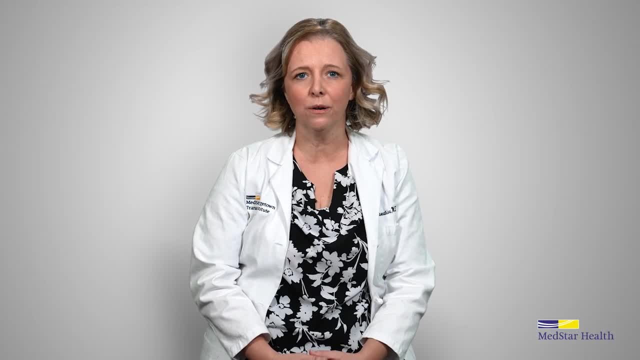 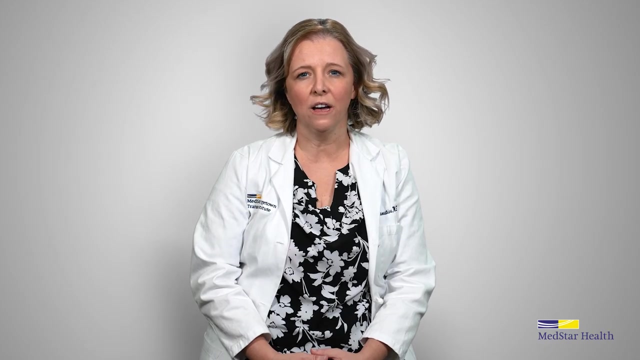 Lack of communication with your coordinator or any member of our transplant team may lead to changing your status to inactive or removal from the waitlist. It is your responsibility to keep your transplant coordinator informed and communicate with us while waiting for an organ. When you are contacted for an organ offer by the on-call coordinator, please listen to what our team asks for you to do. 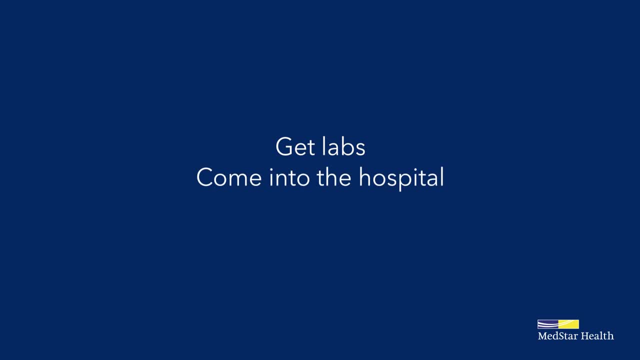 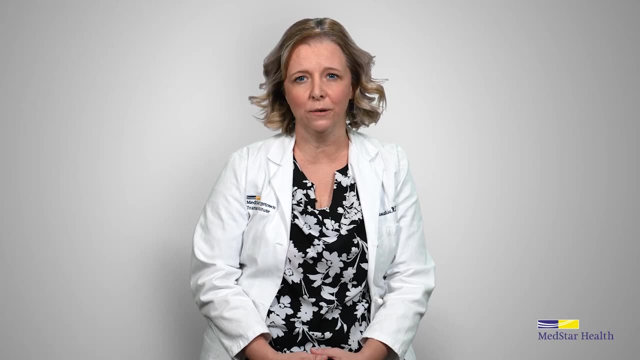 You may be asked to get labs, come into the hospital or simply wait for the next phone call. Please remember: if we can't reach you, we can't offer you an organ. It's also important to remember a potential transplant may be canceled immediately prior to surgery if a donor organ has irregularities, that makes it unfit for you to receive. 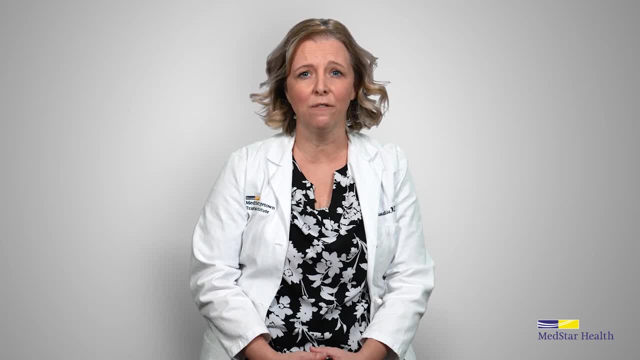 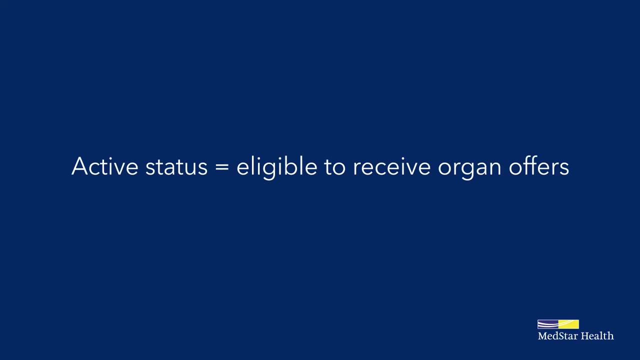 Some final diagnostic testing is done at the time of organ donation. All of these details should be explained. They should be explained to you by the on-call coordinator. if this situation occurs, Active status means that you are eligible to receive organ offers. Inactive status means you are ineligible to receive organ offers, but you are still gaining time on the waitlist.